in all directions, so up and down, And if you read the table, you'll see that the four supplant waves are all on one track of 8 meters per second and then they're all transverse waves In order to make the probability next level, which could be a few, taking back some computers. if you persist another layer, then the first level sequence is just the preserved wave. Once we have all the invisibility left and we class that to thecompressrelativos, which is more or less the only aluminum waveform, then we can call text on the first layer. 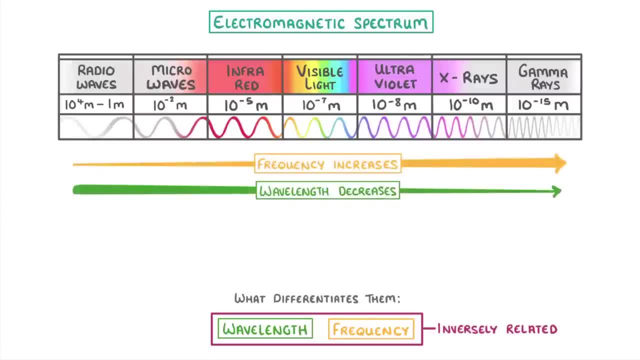 And the frequency increases during sequence While the wavelength decreases. So radio waves have the biggest wavelength but the smallest frequency, and gamma rays have the smallest wavelength but the biggest frequency And to give you a rough idea of the wavelengths they vary from: 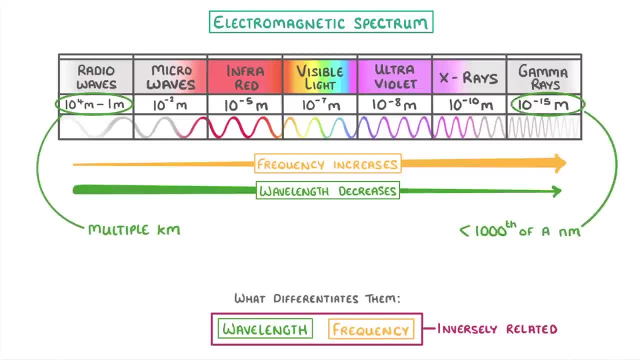 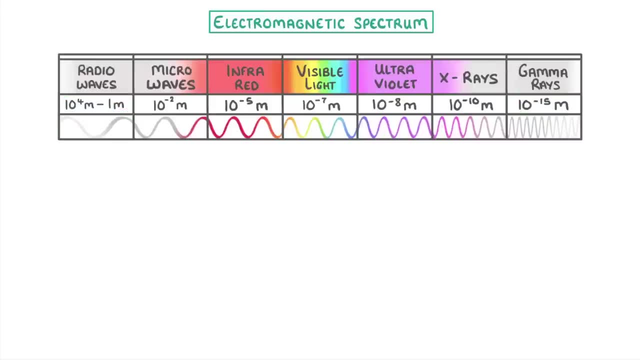 multiple kilometers for radio waves to less than a thousandth of a nanometer for gamma rays. As human beings, though, our eyes are only able to detect a tiny part of the spectrum which we call visible light, and the different wavelengths within this region are what give us all of the different colours that we can see. 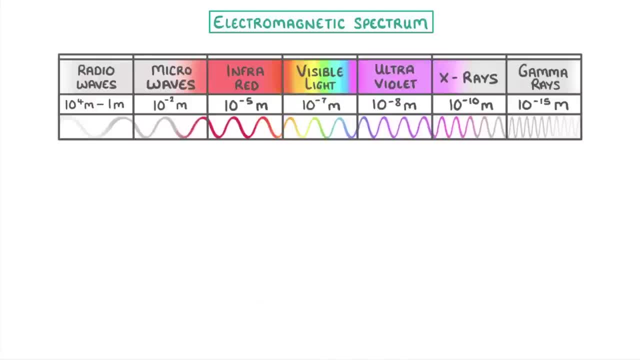 Now, one of these slightly annoying things about this topic is that you need to memorise the order of all the different waves in the spectrum. Personally, I think the best way to do this is to start in the middle with visible light and work your way outwards If you don't know the colours of the 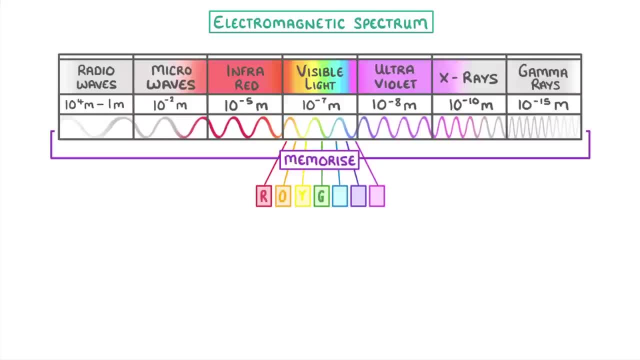 rainbow. already you can remember them as Roy Gee Biff, or red, orange, yellow, green, blue, indigo and violet. After violet comes ultraviolet, which makes sense, and before red is infrared. So I hope you remember that X-rays and gamma rays are over on the right. Remember that all. 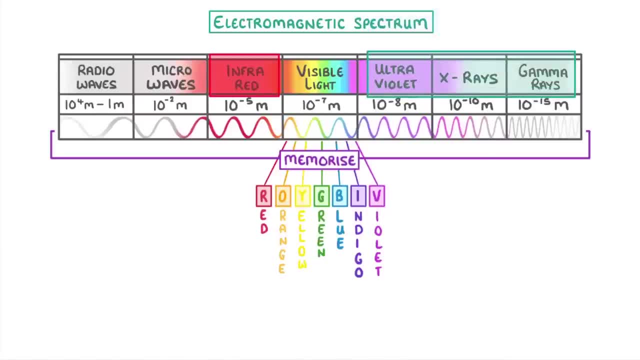 of these types. so ultraviolet, X-ray and gamma can all be ionising and cause damage to our cells, so they're grouped together. Then all we have left are microwaves and radio waves, which are both used in communication and go on the far left.